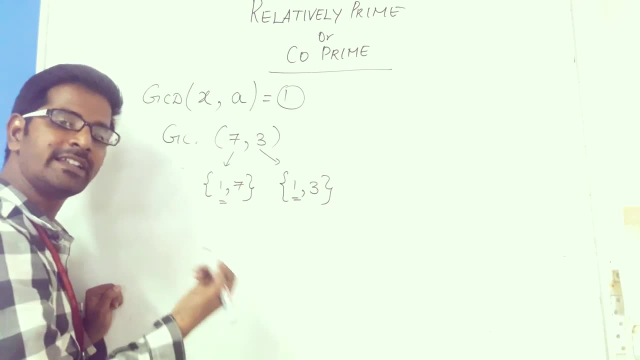 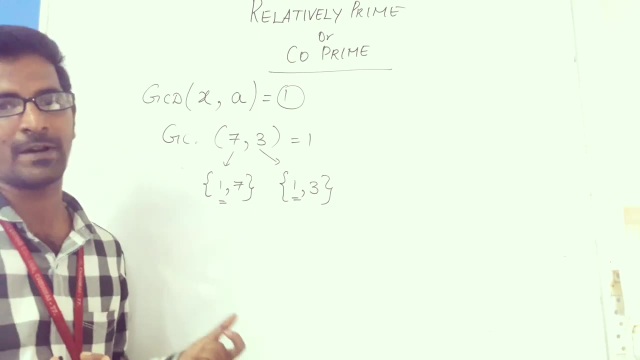 divisor, which is 1, which is 1.. Now we will find out the greatest common divisor, GCD, of 7 and 3, which is equal to 1.. Hence 7 and 3 are relatively prime. So 7 is co-prime to 3, or 3 is co-prime to. 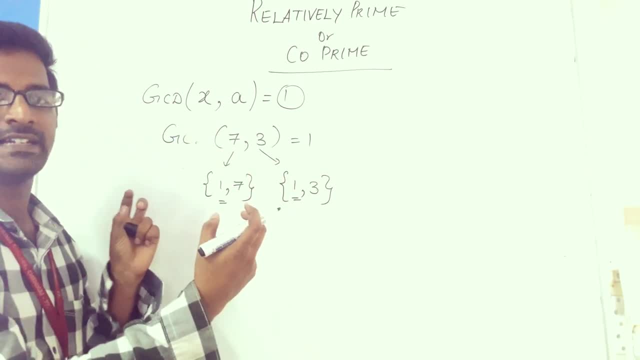 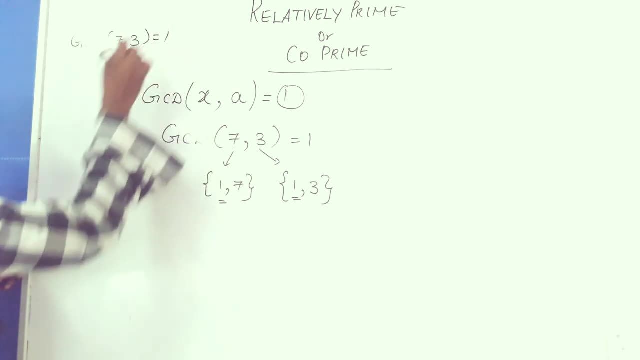 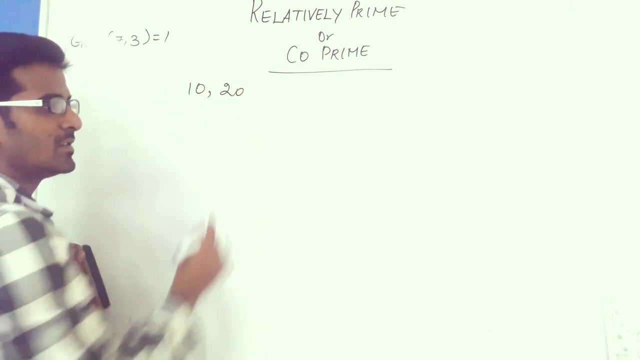 7. So in a nutshell, 7 and 3 are relatively prime. Now we will just make a note of these two numbers. here Let me take 10 comma 20.. Now, when we look at the numbers, we can easily say that 10 and 20 are not. 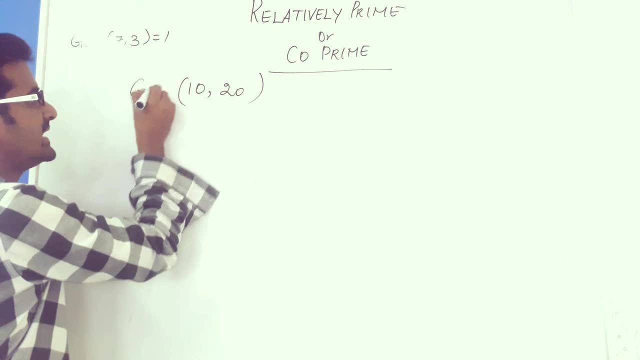 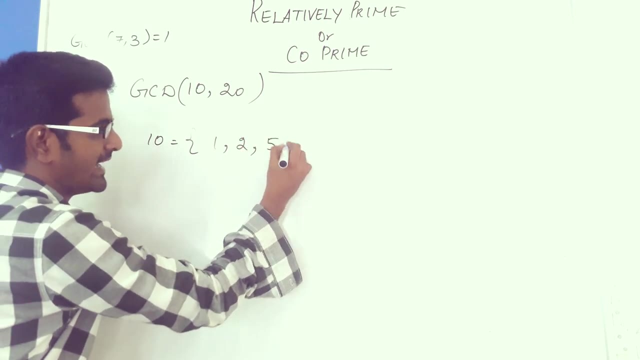 relatively prime. Why? Because the GCD of 10 and 20 should be 1.. We will list out. the devices of 10 are 1,, 2,, 5 and 10.. The devices of 20 are 1,, 2,, 5 and 10.. So we can easily say that 10 and 20 are. 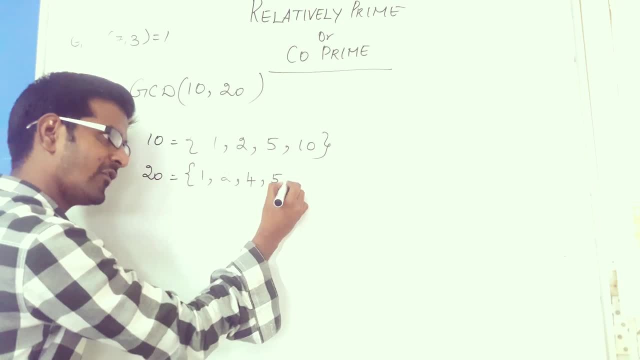 1,, 2,, 5 and 10.. This is wrong. Now, what are the divisors? So 1,, 2,, 5 and 20.. So what are all the common divisors? 1,, 2,, 5 and 10.. getsика. 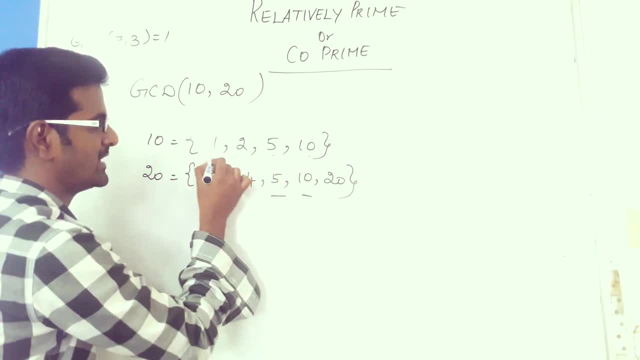 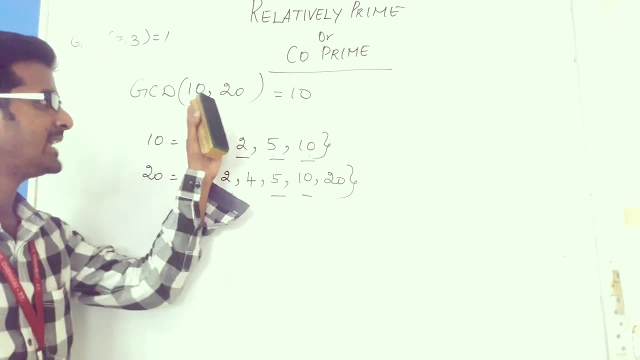 1,, 2,, 5 and 10,. 1,, 2,, 5 and 10,. 1,, 2,, 5 and 10, Now, which is the greatest common divisor? 10 is the greatest common divisor. Hence we can say 10. 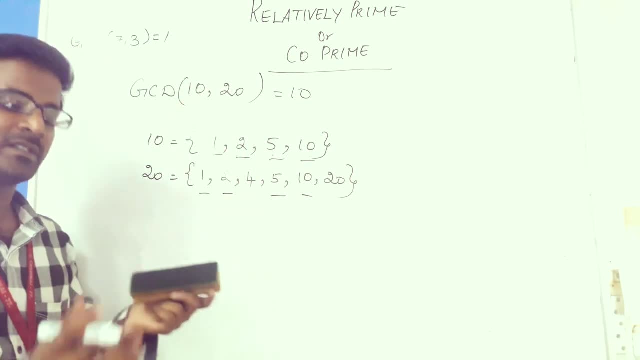 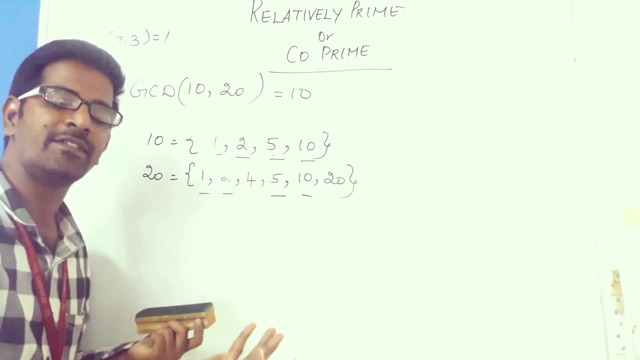 and 20 are not relatively prime, because the concept of relatively prime is when two numbers are relatively prime. If they are not, then it is not prime. So it is not. they do not have any divisors, common divisors, except 1. It means GCD of these two numbers. 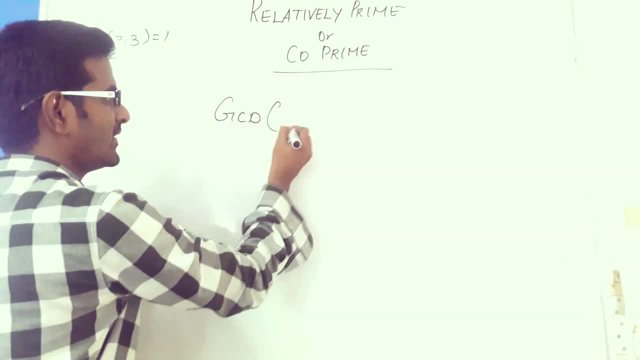 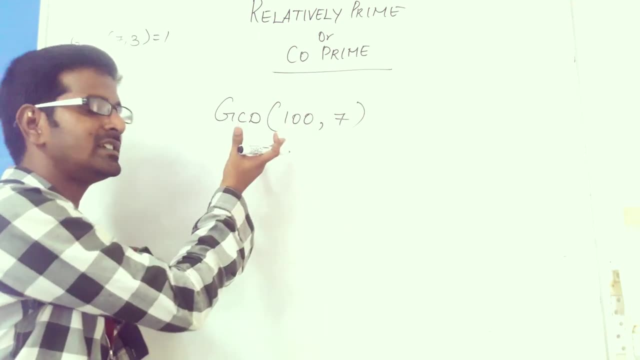 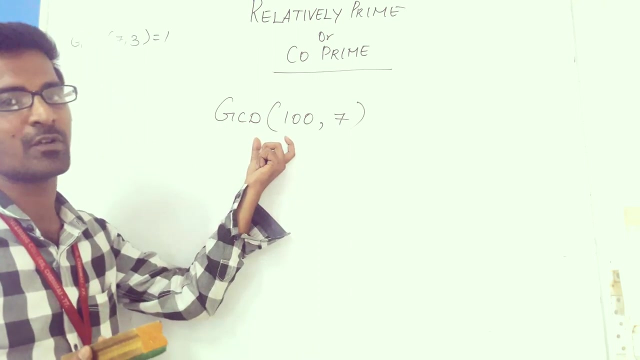 should be 1 GCD of 100 comma 7.. We will calculate the GCD of 100 comma 7.. So for this we can apply Euclidean technique for finding the GCD value, for checking the Euclidean or for doing the Euclidean process, you can refer my tutorial of GCD which gives you some idea. 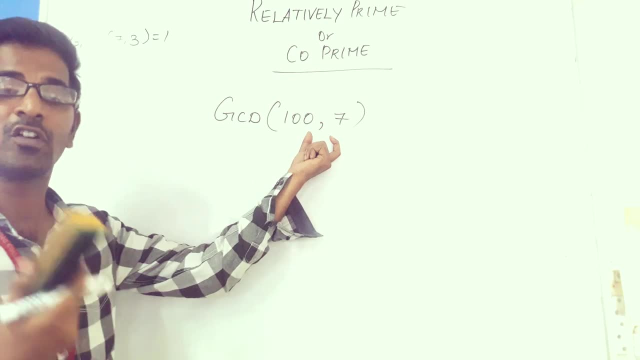 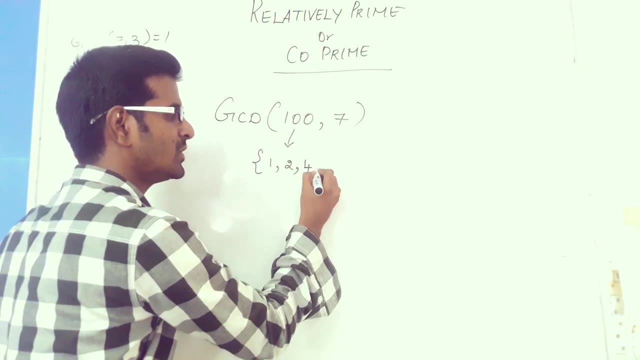 how Euclidean algorithm can be helpful for solving or finding out the GCD value. Now, in this case, just I will list out. the divisors of 10 are 1,, 2,, 4,, 5,, 10,, 20,, 25,. 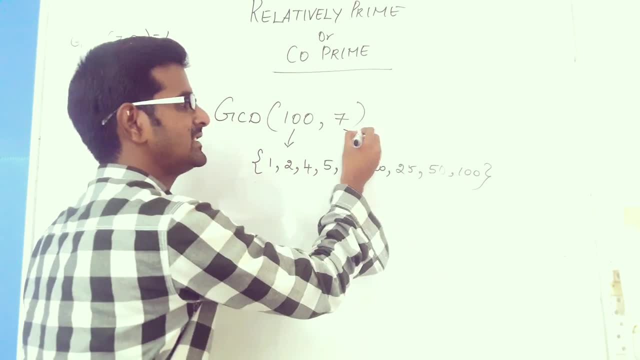 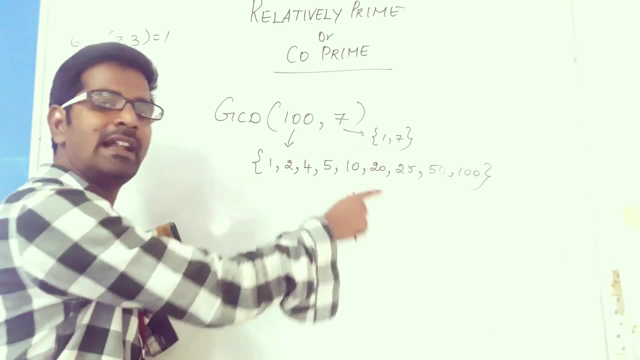 50 and 100.. The divisors of 7 are 1 and 7. because 7 is a prime number, it can have only two divisors. one is 1, another one it is the same number. ok, When you calculate the Euclidean algorithm for finding the GCD value for checking the. 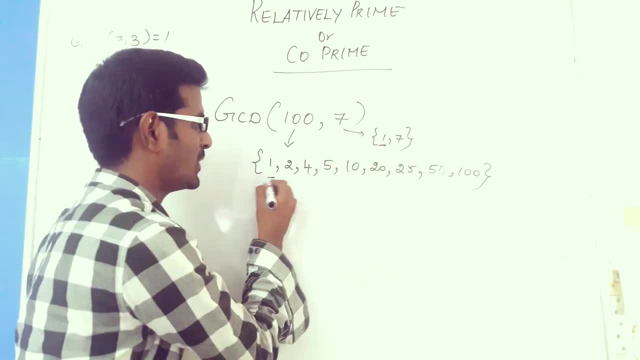 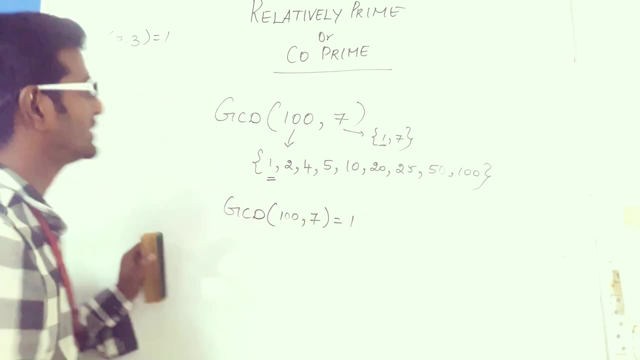 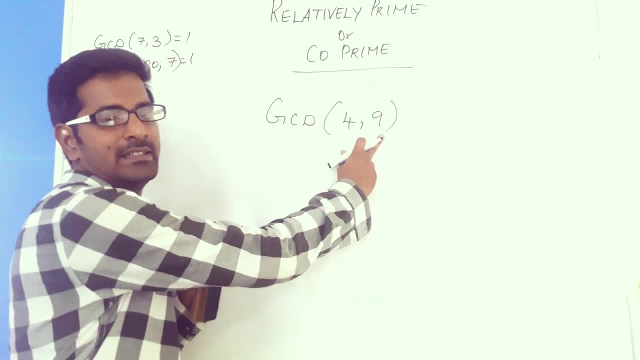 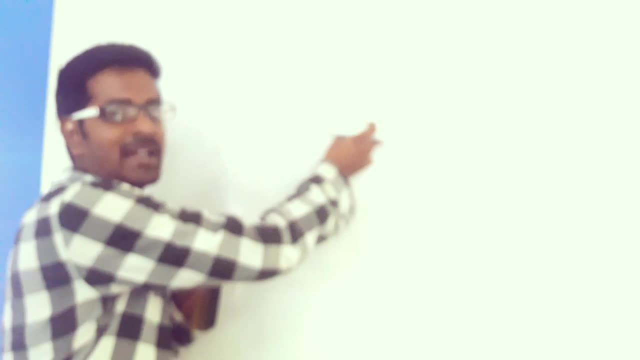 Third example: GCD of 4 comma 9, where 4 is not a prime number and 9 is not a prime number. So I am going to find out the GCD of 4 comma 9, because my intention is: I want to check. 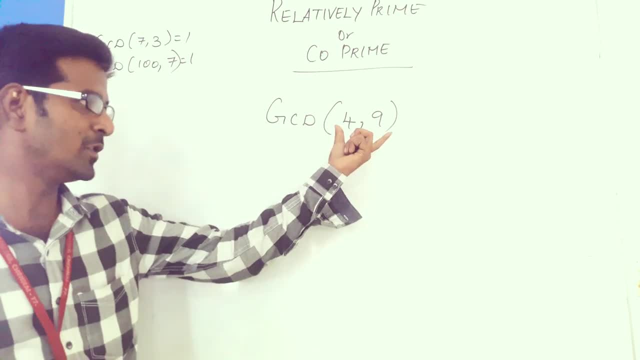 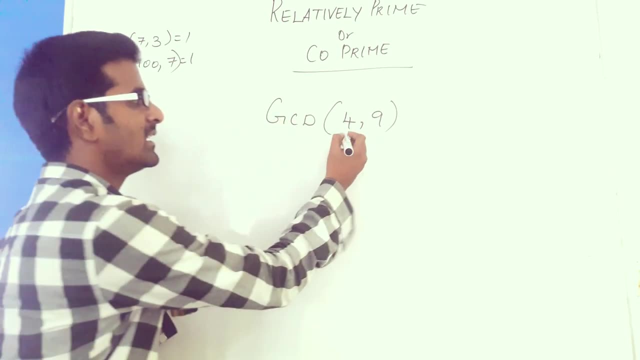 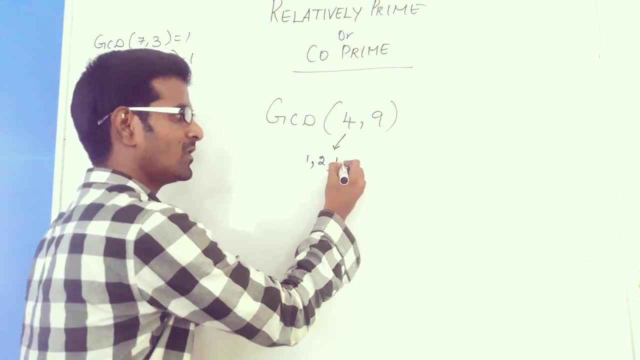 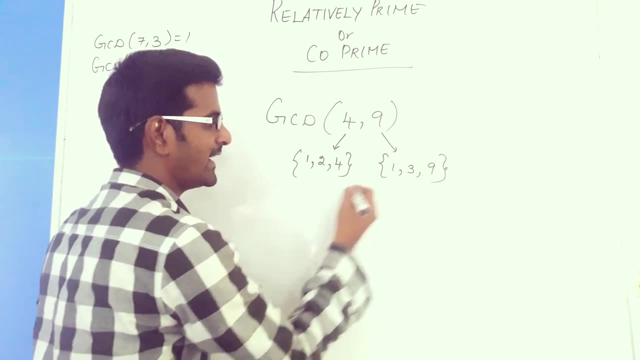 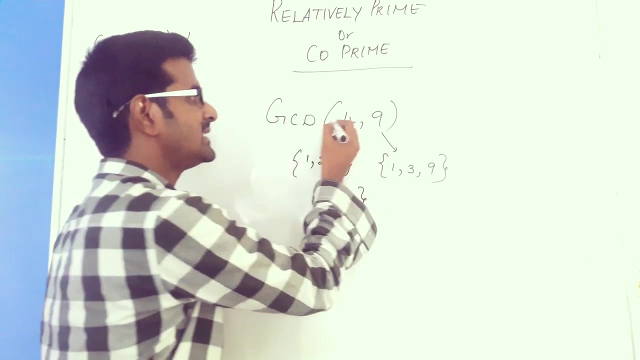 devices of 4? 1,, 2,, 4.. What are all the devices of 9? 1,, 3 and 9.. We will find out the common divisor only 1.. Obviously, this is going to be the greatest common divisor, Hence the GCD of 4,. 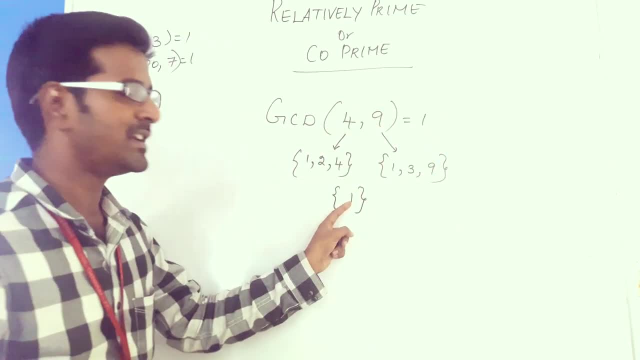 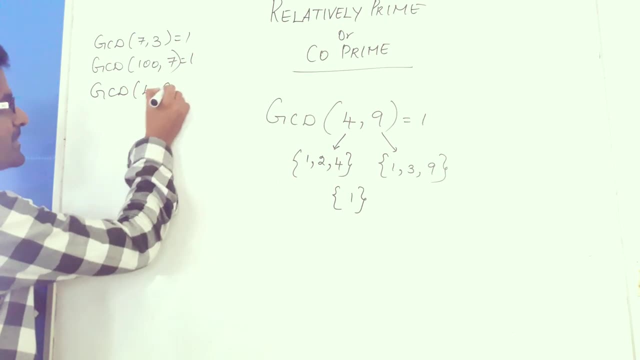 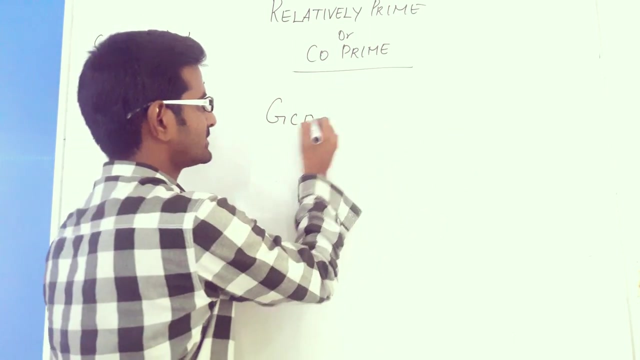 9 is equal to 1, because 1 is the only number that can divide both 4 as well as 9.. So GCD of 4, 9 is equal to 1. ok, The last example. I will just take: GCD of 7, 77. In this case, 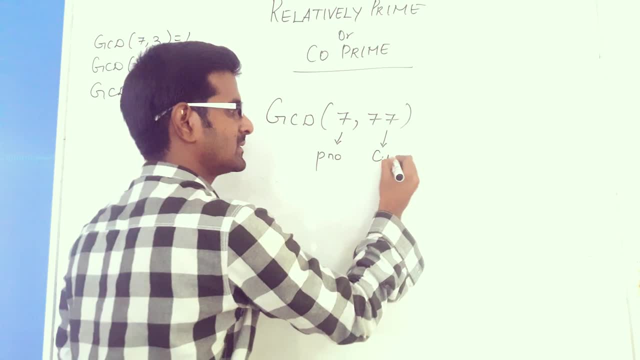 1 is a prime divisor. So GCD of 7, 77 is equal to 1.. So GCD of 7, 77 is equal to 1.. So GCD of 7, 77 is a prime number. 1 is a composite number. A number which is not a prime number is a. 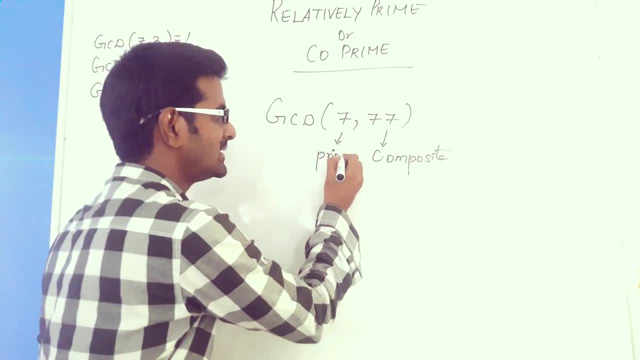 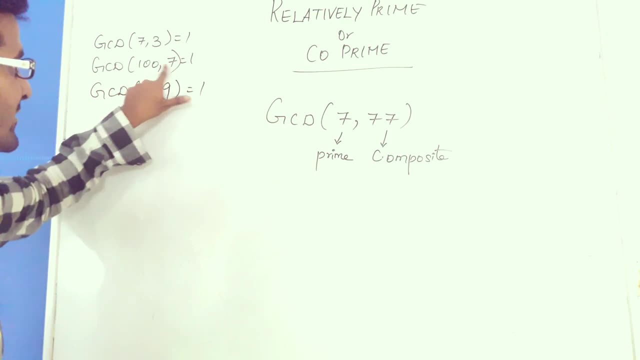 composite number. ok, So now this is a prime number. ok, Now we will see. already we have taken one example. Just see here: 100 and 7.. In this case, 100 is a prime number, 100 is a composite number, 7 is a prime number. So we, we we confirm that these two numbers are. 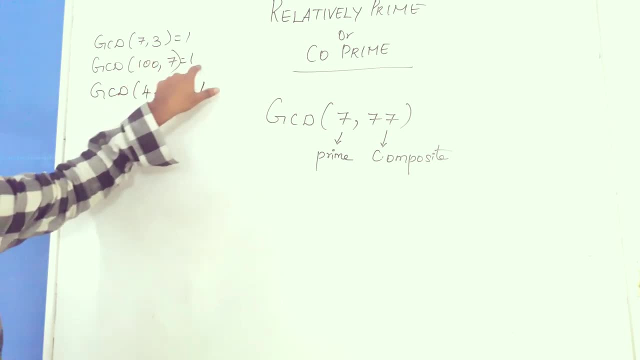 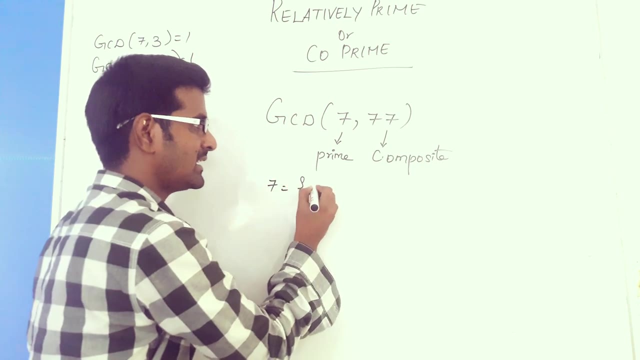 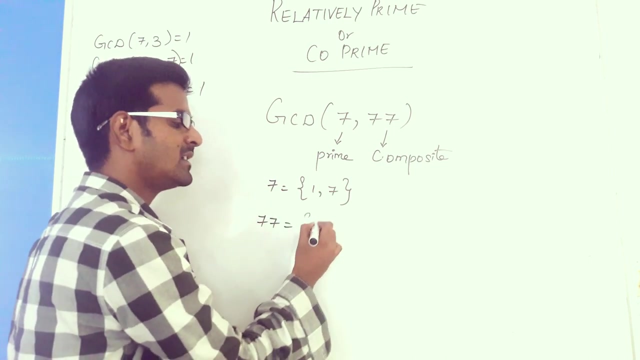 relatively prime, because the GCD of these two number gives only 1 right. Now we will find out the. we will calculate the GCD of 7 and 77. The divisors of 7 are 1 and 7. since it is a prime number, we can have only two divisors. Now. the divisors of 77 are 1, 7, 11. 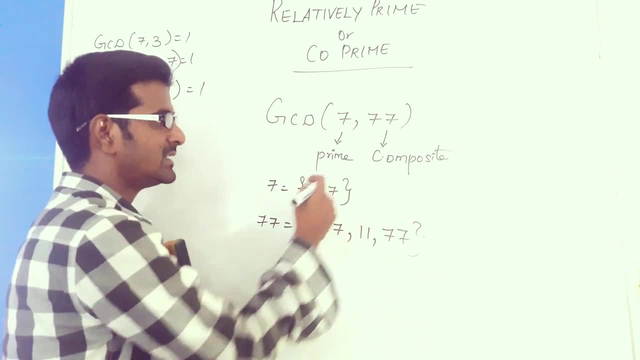 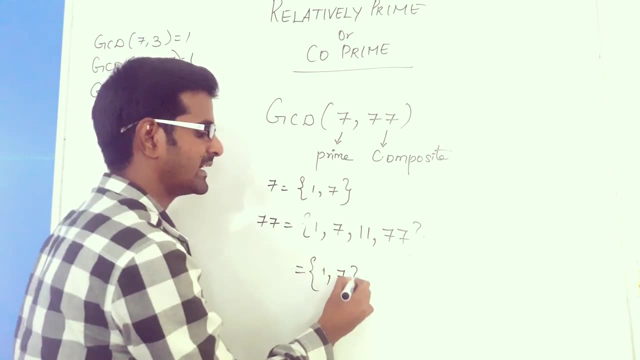 and 77. Now we will find out the GCD of these two numbers, The common divisors we will list out. So 1 is common in both the case. 7 is common in both the case. Now, which is the greatest number, 7 is. 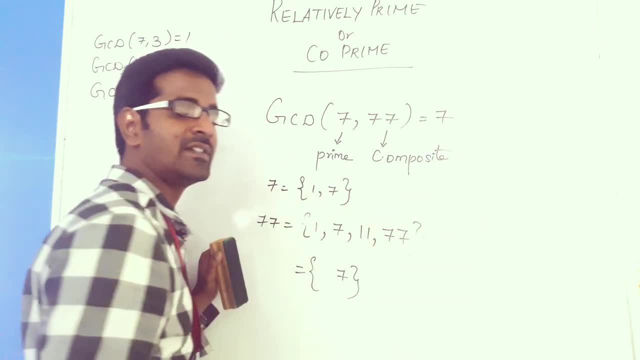 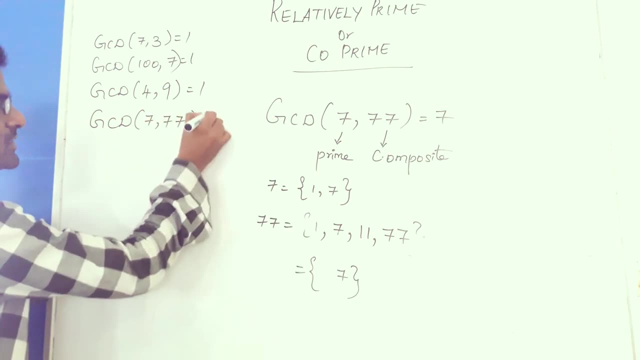 the greatest number. So GCD of 7, 77 is the greatest number. So GCD of 7, 77 is the greatest number. So GCD of 7, 77 is equal to 7.. So I will just list out: GCD of 7, 77 is equal to 7. 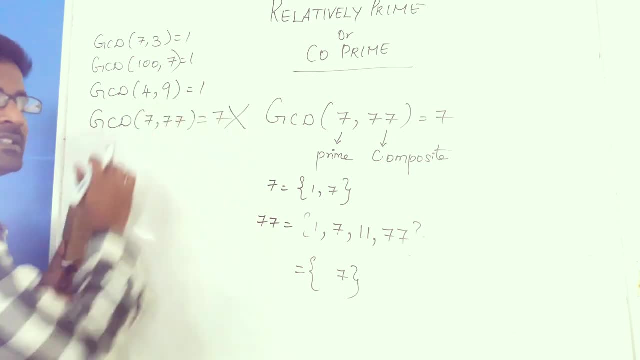 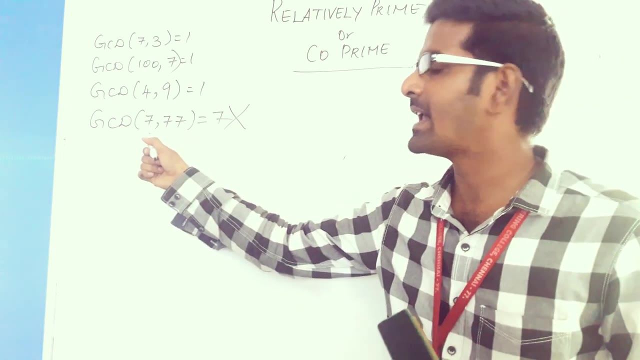 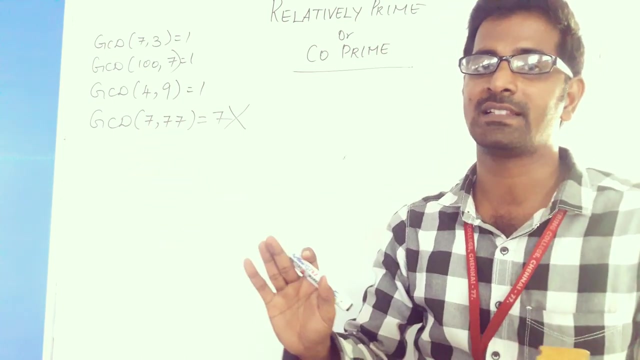 ok, So here this is not a. these two numbers are not relatively prime. So when we look at the scenarios, ok, some people will get confused, right? When one number is a prime number in a GCD operation, definitely we will. these two numbers are relatively prime. It is not like that, Just. 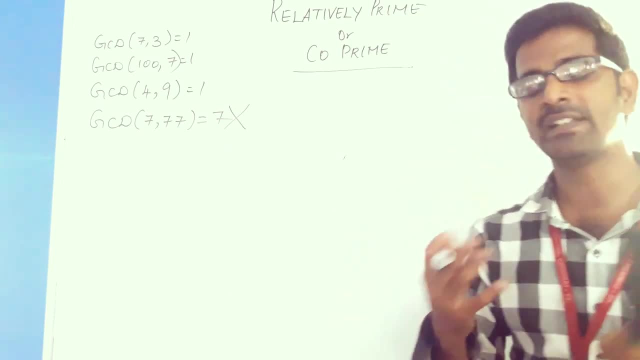 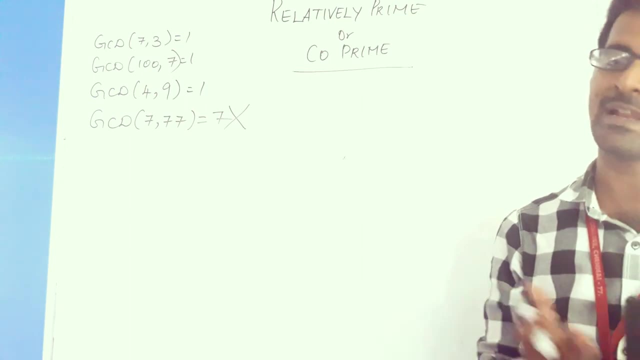 I will just provide. When we are going to calculate or when we are going to find whether the given two numbers are relatively prime, we have to find the GCD of these two numbers. If these two numbers are prime numbers, obviously we can darely say the GCD of these two numbers are. 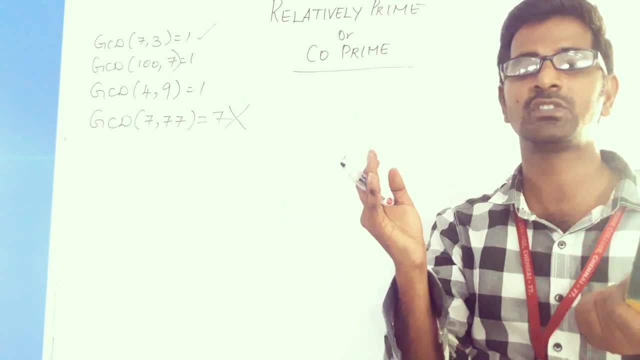 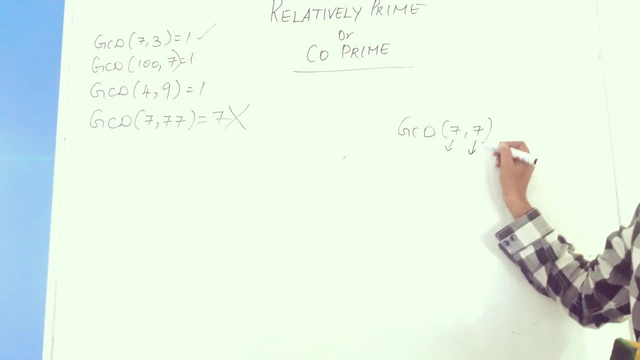 1, and only one condition is that these two numbers should be different. For example, GCD of 7 comma 7, this is a prime number and this is still a prime number. So we will get 7 only, not 1, ok, So. 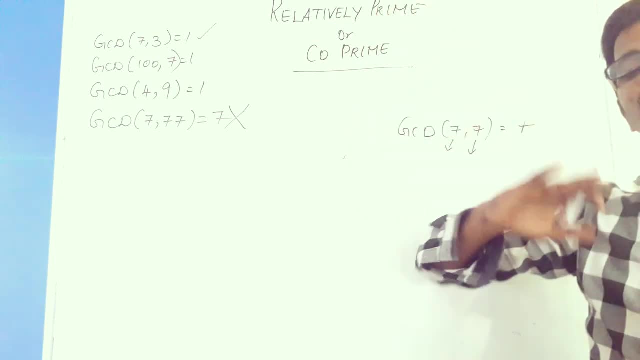 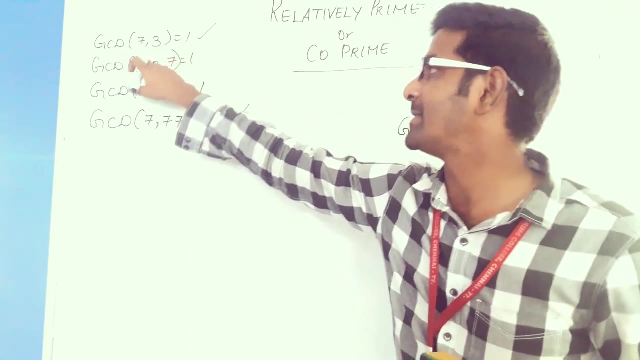 we are going to check whether the given numbers are relatively prime. these two numbers should be different, ok, So in this case, one is a prime number, another one is a prime number. So both are prime number, hence they are relatively prime. The second example, one is a composite number.